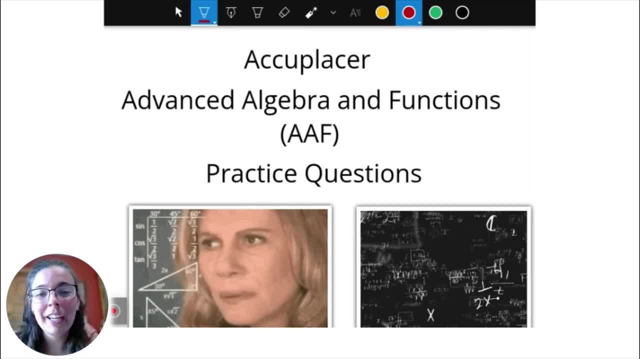 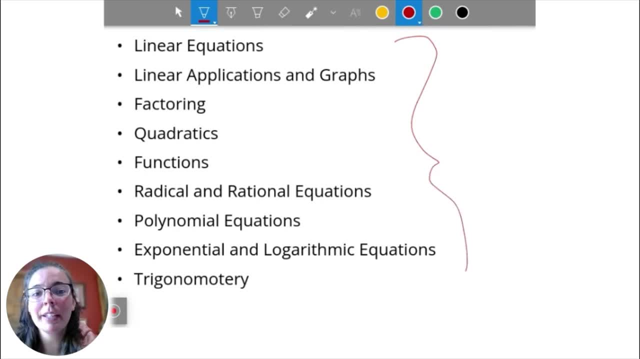 Okay, so let's jump into it. today, We're going to have some practical examples of what you might see on this exam, So here's what we're going to go over today. All right, these are the topics that are on the AAF section of the ACCUPLACER exam. So we're 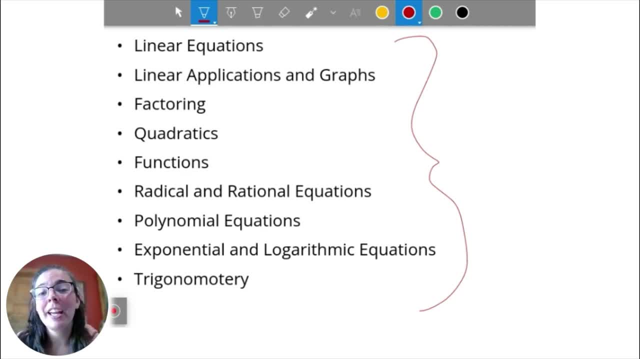 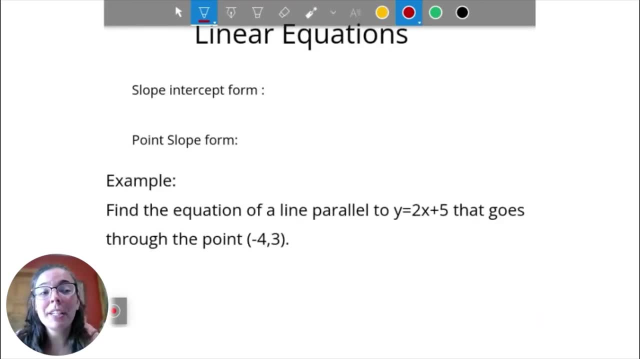 going to go through. I'm going to give you some tips about each section, each topic in the section, and we're going to do an example problem. Okay, so linear equations: A couple things we need to know with linear equations. So important that we know slope. 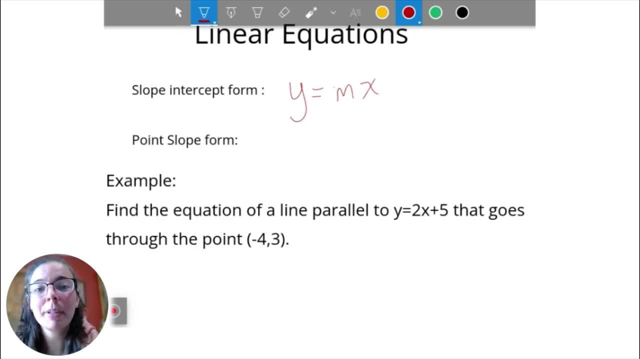 intercept form, which is y equals m, x plus b, where our m is our slope and our b is our y intercept. Also important to know is point slope form: y minus y1 equals m and then in parentheses, x minus x1.. So this is where we have our slope and then we can plug in a point x and y. Okay. 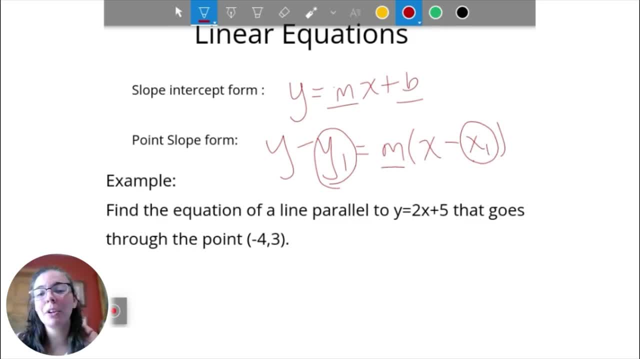 we plug it into our x1,, y1, and then we can solve. So, depending on the question, you would have to use one of these different formulas for our line. So let's look at an example. Find the equation of a line parallel to y equals 2x plus 5 that 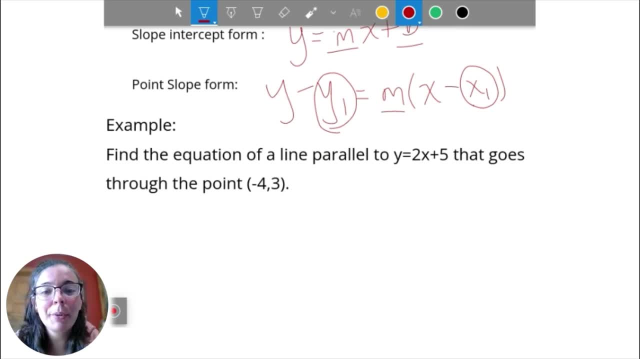 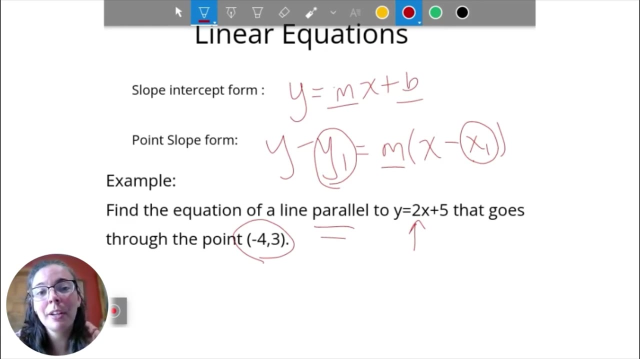 goes to the point negative 4, 3.. So a couple things we need to know here. A parallel line has the same slope, So we already know our slope, and it goes to the point negative 4, 3.. do this We could either plug into our y equals mx plus b. We'd have to go find the y-intercept. 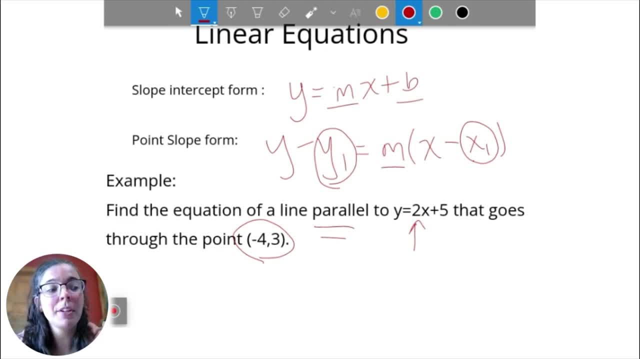 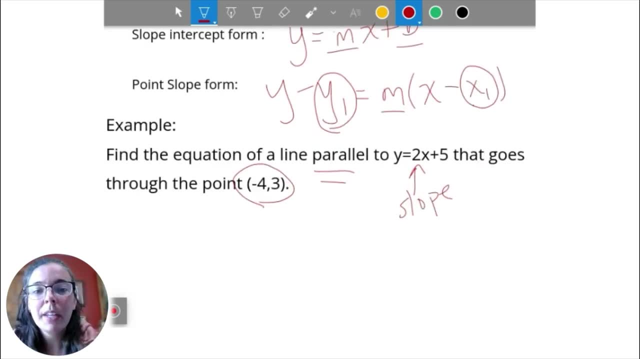 or we could plug into our point-slope form. So for this example it actually seems easier because we know our slope and we know a point. So if I go ahead and plug this in y minus y1, so that's our y value of 3, equals the slope, which is the same, so that's 2, times x minus and then our x value. 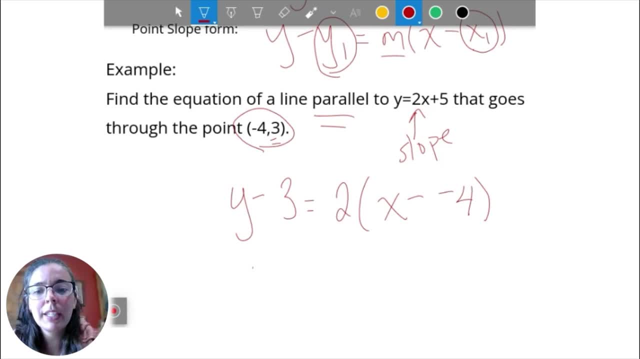 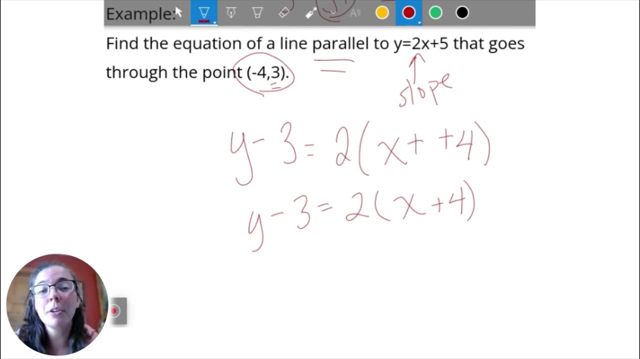 is negative 4.. So minus a negative 4. We could clean this up a little bit by just knowing that minus a negative is actually plus. So this is the equation of our line. but if, say, we needed to plug this into our y equals in order to graph it, our slope-intercept form is better for that. So we 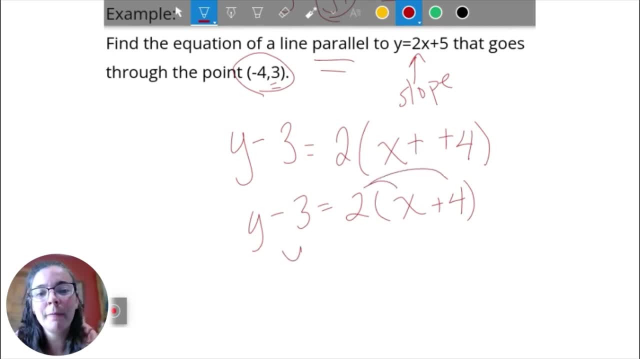 can actually convert straight from here by distributing, and we get 2x plus 8, and then add 3 to both sides to move that over And we get 2x plus 11.. So you also could have done this using slope-intercept form, but for the way 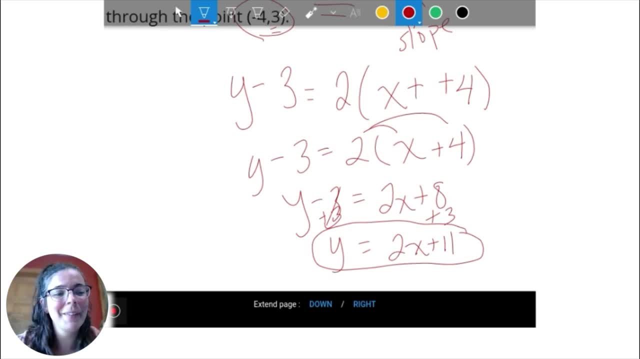 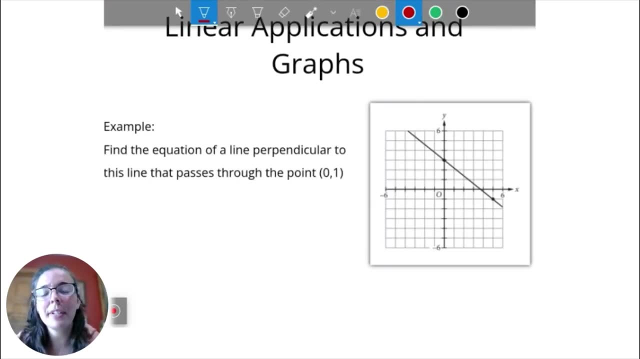 this question was worded. this one was actually a little bit easier. Okay, so that's just an example of what you might see in your linear equations section. There also is linear applications and graphs, So let's look at a couple of those examples. Find the equation of a line perpendicular. 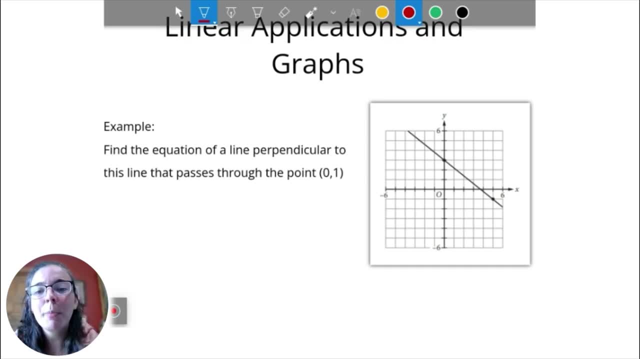 to this line that passes through the point 0, 1.. So perpendicular lines do not have the same slope. They actually have slopes that are negative reciprocals. Okay, so what that means is we find the slope of this line, which we can do by going 1, 2.. Let's see. what do we have to do Actually? 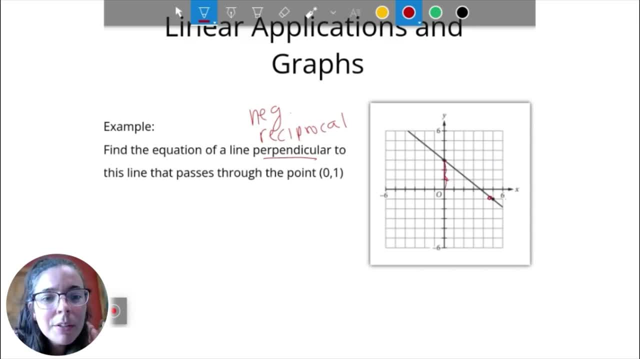 1, 2, 3.. Oh, here's the point, Sorry. Go 1,, 2,, 3, 4.. Go down 4, and then go over 1,, 2,, 3,, 4, 5.. 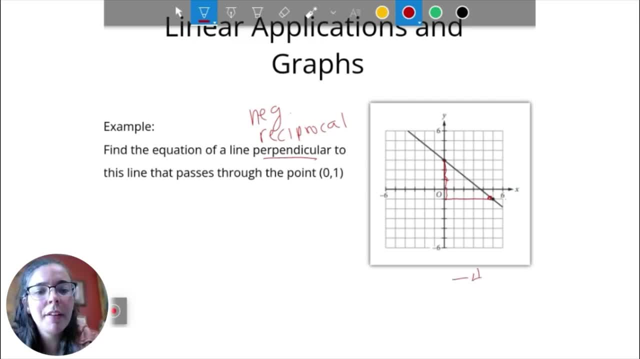 So the slope of this line is down: 4 over 5.. So that can be represented by negative, Negative, 4 over 5.. Now to turn that into the negative reciprocal, we're going to flip it and make it positive. So our new slope is going to be positive: 5 over 4.. And now this goes through the 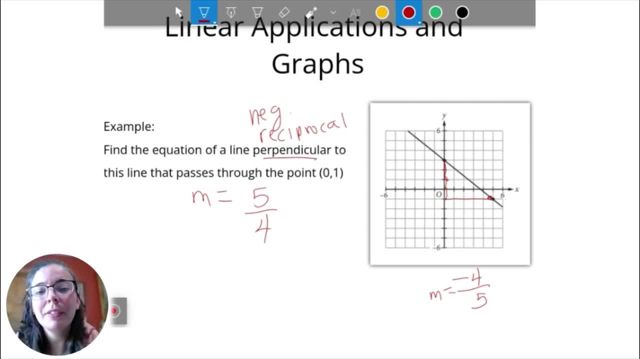 point 0, 1.. So two things that we could do. We could either plug it into our point-slope form or our slope-intercept form, So they give us a point of 0, 1.. Okay, so that means over 0, up 1.. 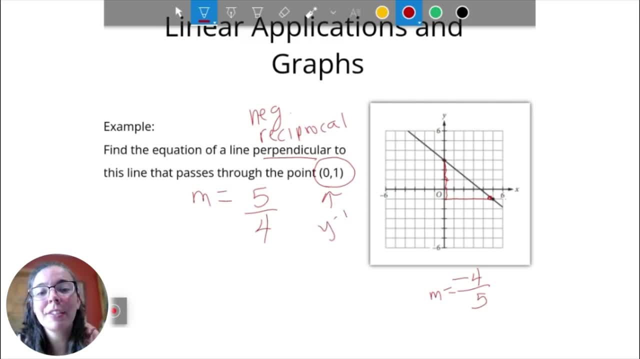 So that's actually our y-intercept that they gave us. Our y-intercept here is b equals 1.. So I'm going to use y equals mx plus b and plug in my new slope and then my y-intercept of 1.. Okay so, taking a graph and 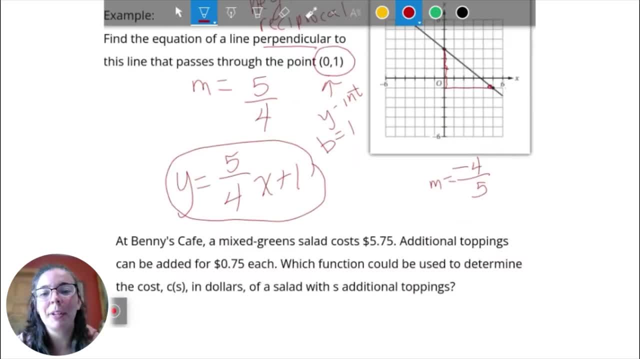 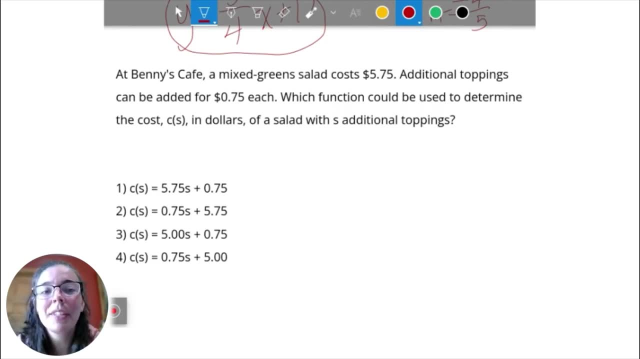 figuring out the equation of a line that's perpendicular to it. Here's an application problem. At Benny's Cafe, a mixed green salad costs $5.75.. Additional toppings can be added for $0.75 each. Which function of the equation do we use? We use the function of the equation. 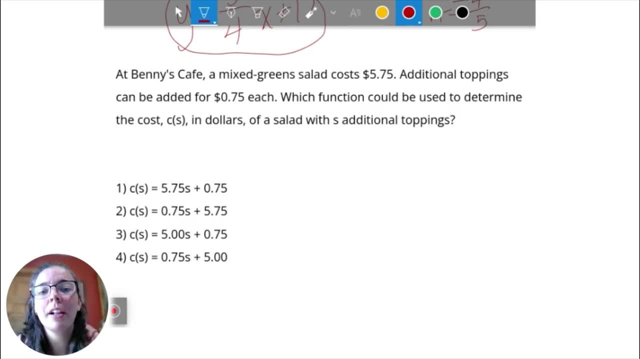 to determine the cost c of s in dollars of a salad with s additional toppings. So here we need to figure out- notice how all of our answers follow this- y equals mx plus b form. So from this application problem we need to figure out which one is our slope and which one is our y. 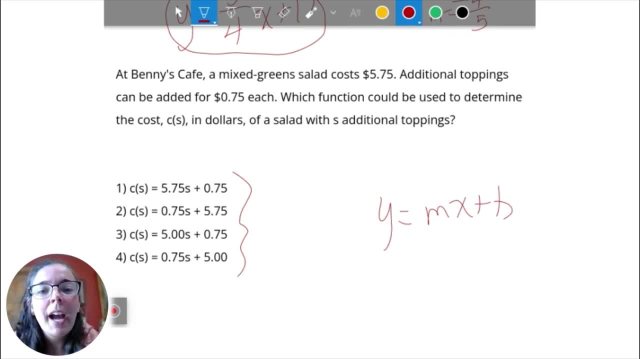 intercept, so to speak. So it costs $5.75, and then for each additional topping it's $0.75 each. So that represents the toppings. So s here right, all of the s's should be multiplied by $0.75.. So I 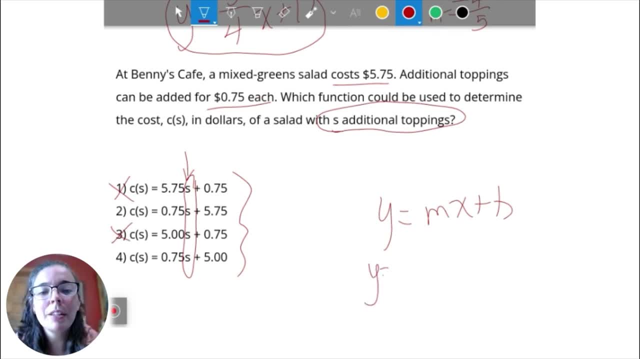 can actually get rid of 1 and 3.. So I know that my slope is $0.75.. Okay, and then my y-intercept is how much it costs initially for the salad, which is $5.75.. So if I match this up with the 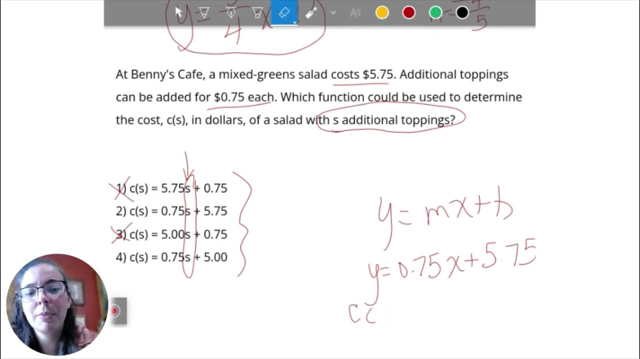 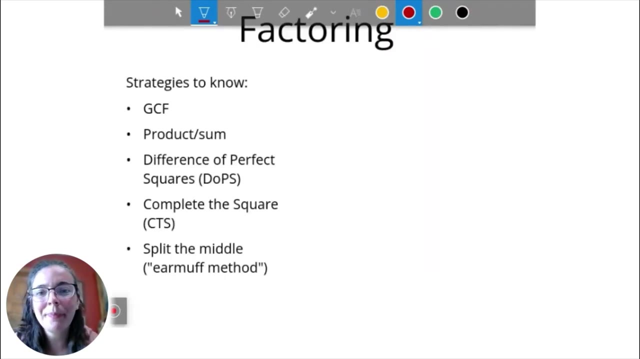 appropriate function notation. sorry, that should be c of s. that would equal $0.75.. 5s plus $5.75, which looks like option number two. All right, our next topic is factoring. So factoring is a big topic. You're going to need to really be comfortable with lots of different. 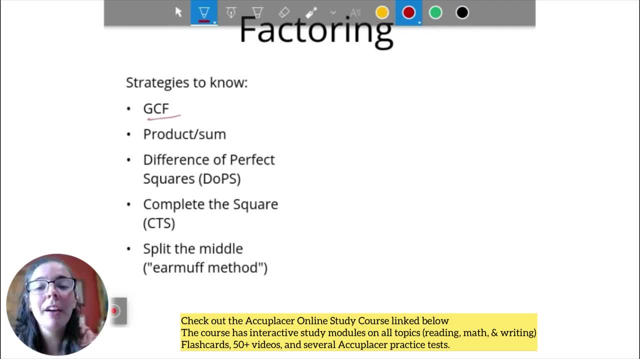 strategies. So strategies to know We can pull out the GCF of something. Say we have like 3x plus 6 and we need to factor it. All we have to do is pull out the 3 and then we're left with x plus 2. 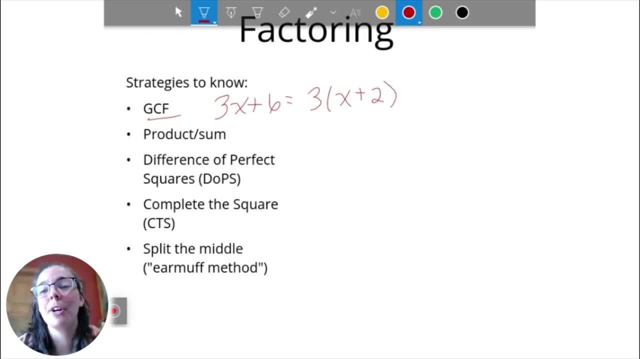 in factored form. Okay, it gets more complicated when we're dealing with quadratics and bigger numbers, but it's important to always check for your GCF. to start, Product sum method is really good when we have something like x squared plus, let's say, 3x plus 2.. Okay, product sum method. 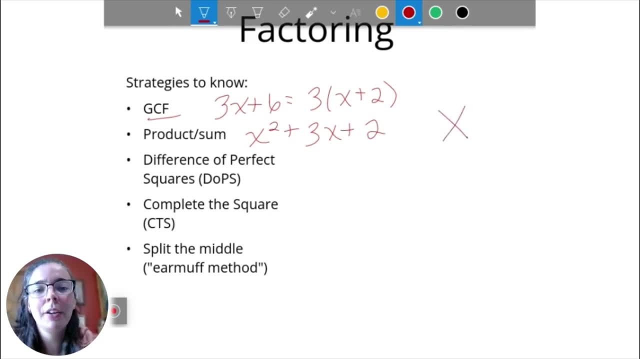 which we will practice in an example later, basically tells me: well, I know it needs to multiply to 2 and add to my middle term of 3.. So I can figure out my factors that way. In this case it would be 1x. So I can figure out my factors that way. In this case it would be 1x. So I can. 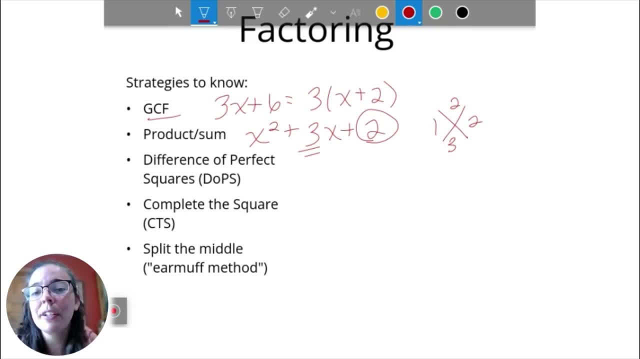 figure out my factors that way. In this case it would be 1x, So I can figure out my factors that way. Difference of perfect squares, or DOPs, is great when we have a binomial that looks something like this: x squared minus 16.. So x squared and 16 are both perfect squares And the difference comes in. 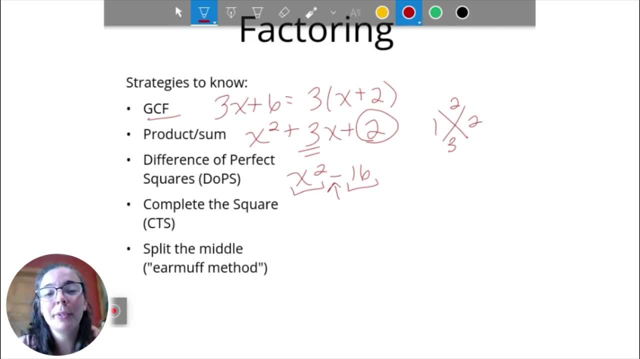 here with a minus sign. So there is a strategy in order to factor that Completing the square is really helpful if we have something that doesn't factor, using the product sum method very easily, So then we can complete this And then, last but not least, split the middle, or what I call the earmuff method, is really helpful. 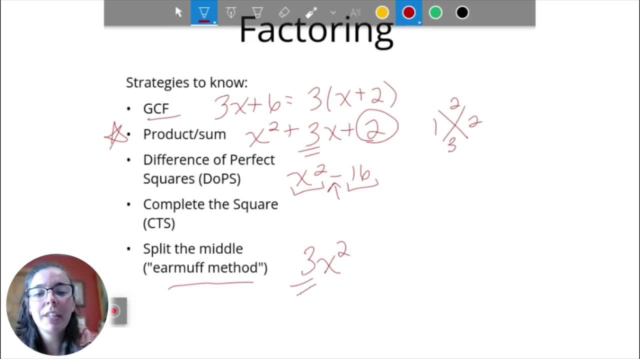 if we have a coefficient in front of the x squared, So maybe it's something like this. Okay, so all of these strategies are really helpful. If you want a more in-depth video about any of these strategies, leave me a comment so that I can come back and I can do videos. 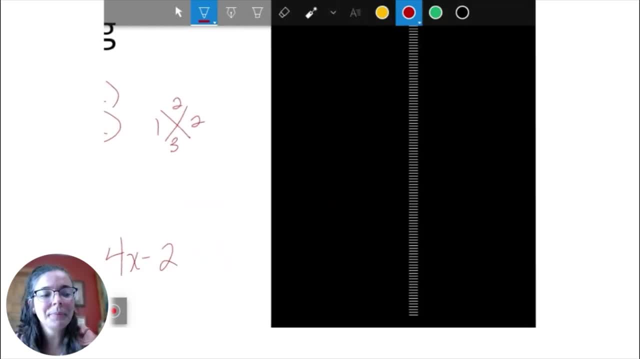 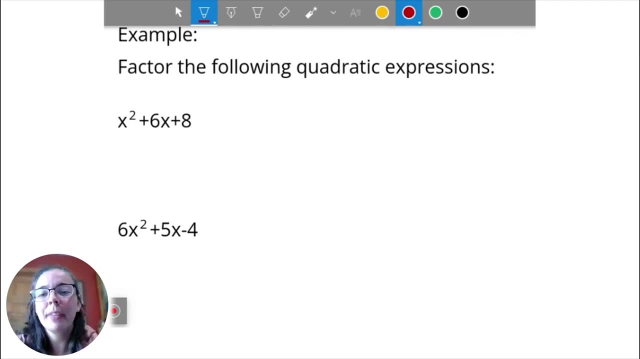 that really dive into each of these different topics. So here's a couple examples. So we're going to do x squared plus 6x plus 8.. So if I'm going to factor this, this is a good example for the product sum method. So I draw my x And when I'm factoring I need it to multiply to 8 and add. 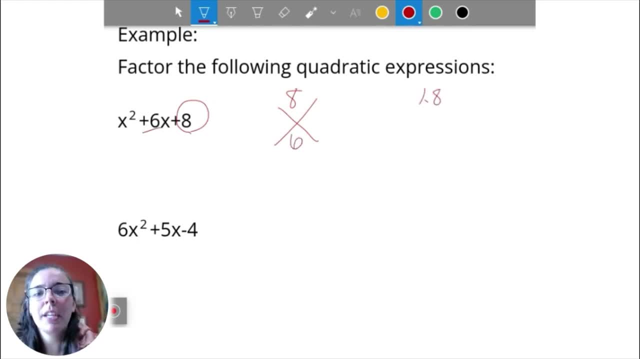 to 6.. So factors of 8 are 1 times 8 or 2 times 4.. So the ones that add to 6 is 2 times 4.. They can both be positive, because 2 times 4 is 8 and 2 plus 4 is 6.. So what I do is I draw my parentheses. 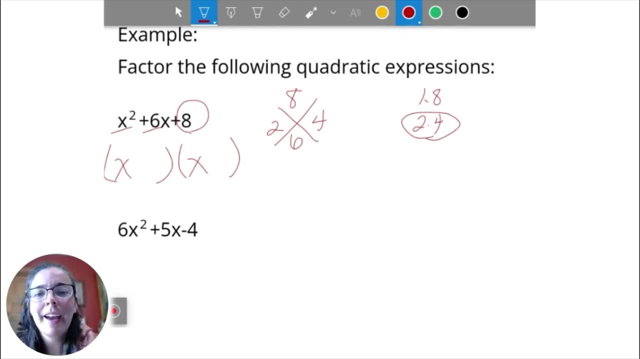 The x squared gets broken down into two. So I'm going to do x squared plus 6x plus 8.. And I'm going to broken up into x times x, And then my factors I just found are plus 2 and plus 4.. So that is my. 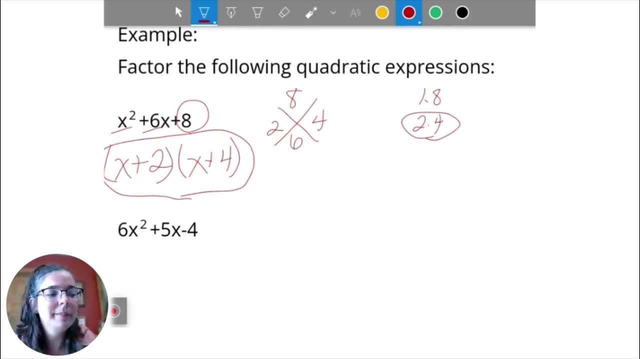 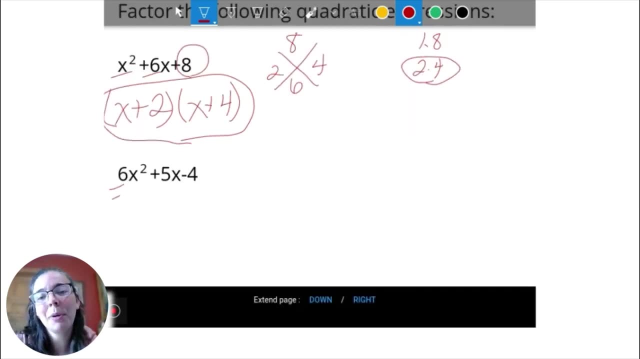 factored form of that expression. So that's great. What happens if I need to do something like split the middle because I have a coefficient in front? Okay, so it's going to be a similar process, But I call this the earmuff method because I actually have to take the 6 and the negative 4. And I have 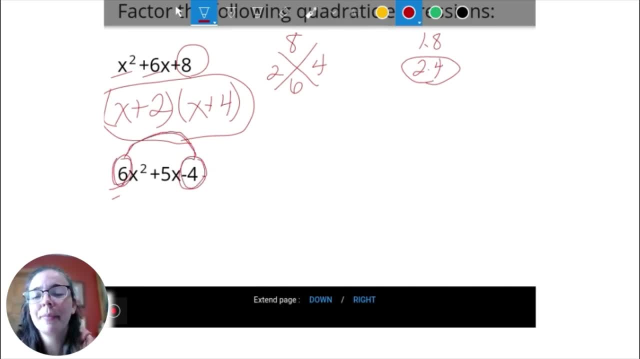 to multiply them. So notice how it kind of looks like some earmuffs. So 6 times negative 4 is negative 24.. So I need it to multiply to negative 24 and add to 5.. So factors of 24 are 1 times 24,. 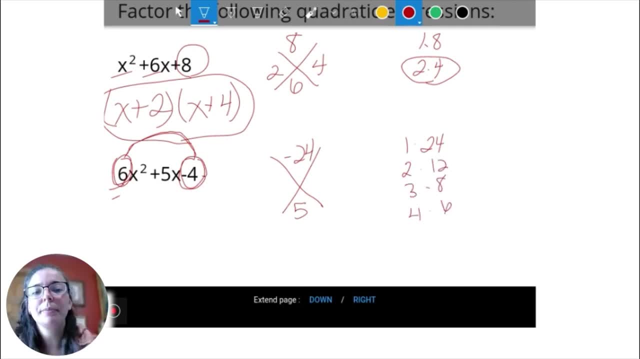 2 times 12,, 3 times 8,, 4 times 6.. The only one that has a difference of 5 is 3 and 8. So I need it to add to a positive 5.. So I need the 8 to be positive, and then the 3 can be negative. 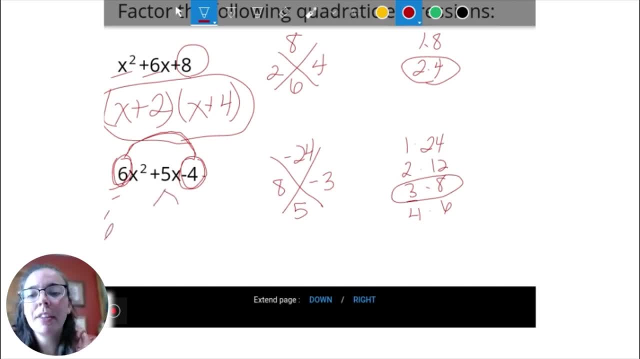 So what that allows me to do is split the middle. So I'm going to rewrite this as 6x squared, and the 5x I'm going to rewrite as plus 8x, minus 3x- That's what these were for, Minus 4.. And now I can. 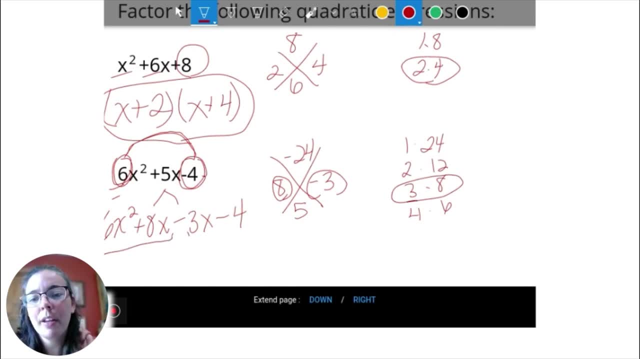 just split these into two separate sets of terms to find the GCF of. So 6x squared and 8x, I can pull out a 2x and I'm left with 3x plus 4.. And then negative 3x minus 4 only has a GCF of a. 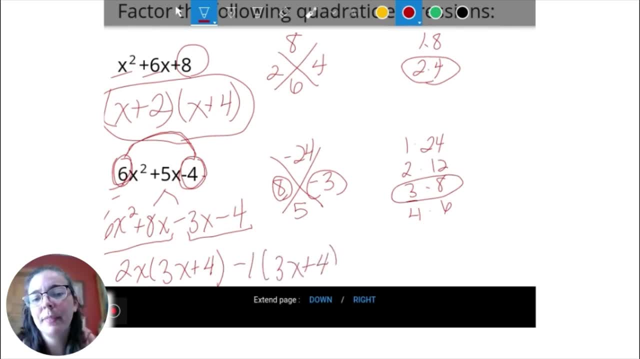 negative 1.. So I'm going to pull that negative 1 out and get 3x plus 4.. So I'm going to pull that negative 1 out and get 3x plus 4 here. And that's key, because I need to have the same thing in my. 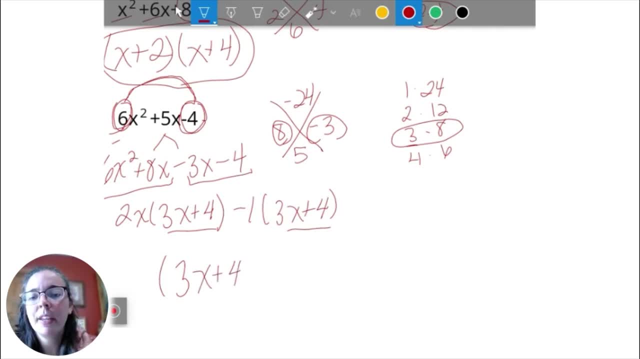 parentheses. So I pull that out: 3x plus 4.. And what's left over is 2x minus 1.. Okay, So we factored that using split the middle. Again, if I'm going a little bit fast for you and you're, 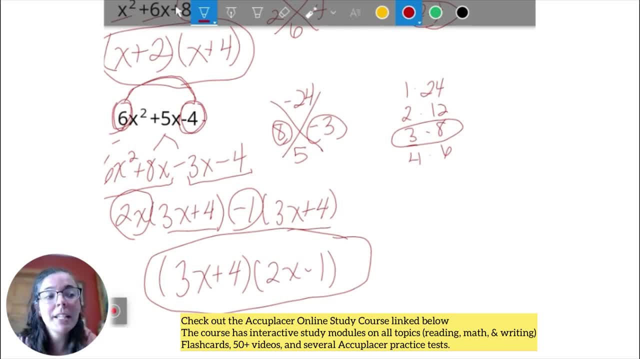 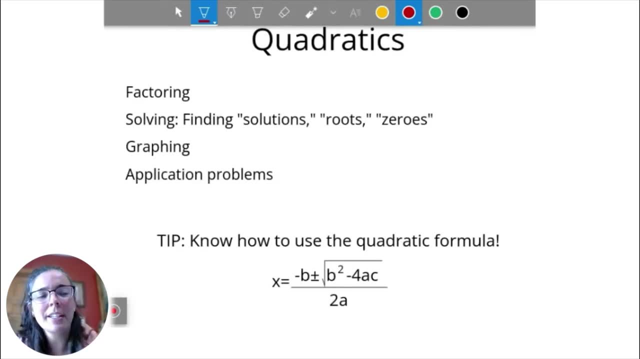 like: oh, this is like kind of a tricky topic. I need a little more support with this. Please leave me a comment. I can go over this in a lot more depth and not so quick if you guys need it. So our next topic is along the same lines, with quadratics, One thing that we can do with. 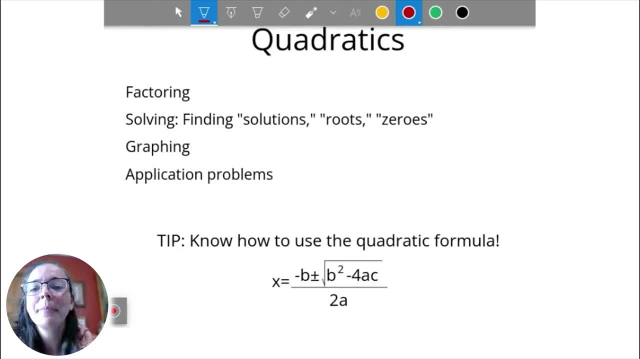 quadratics is factor right, So we can factor. We just practice that a little bit. We also may need to solve- or sometimes we see that as finding solutions- roots or zeros. We may also need to graph or do application problems of your quadratics. So a big tip I have for different quadratics is: 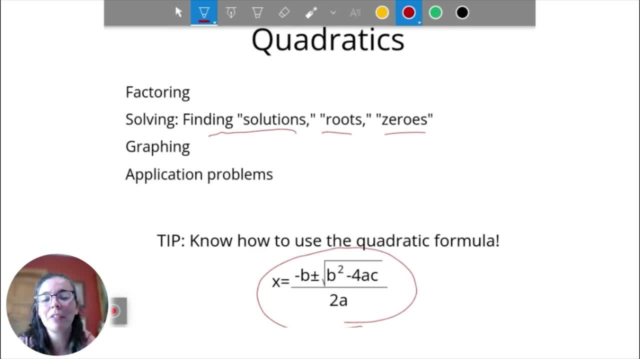 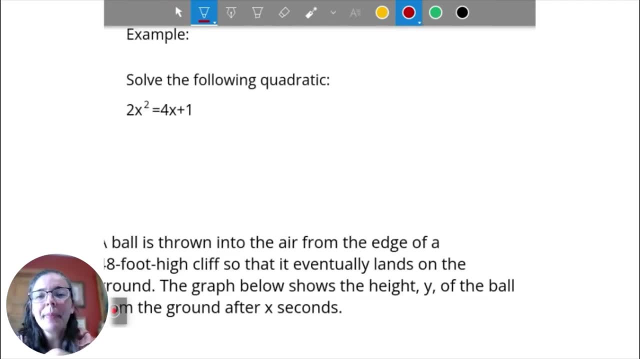 know how to use the quadratic formula. Okay, So this quadratic formula can allow you to find solutions for any quadratic equation. So if you have a quadratic equation, you can use the equation. So let's look at a couple examples. Let's solve the following quadratic 2x squared. 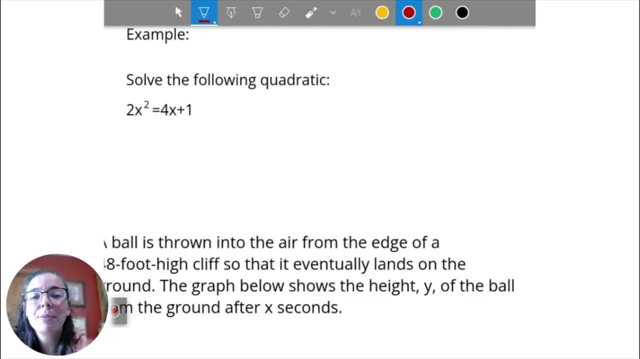 equals 4x plus 1.. So, in order to do this one, let's practice the quadratic formula. So x equals negative b plus or minus the square root, b squared minus 4ac, all over 2a In order to figure out, 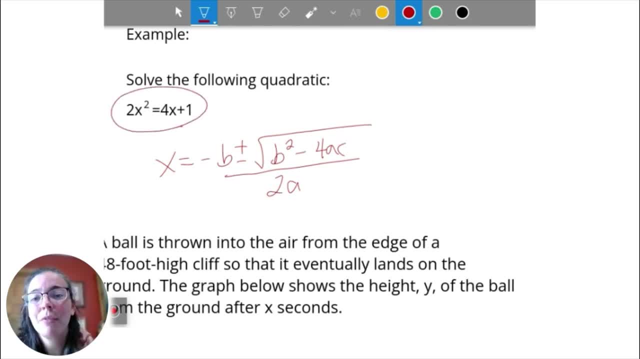 well, what is my a, b and c? I need this to be in standard form, So I'm going to move everything over to the left. 2x squared, it would be minus 4ac, So I'm going to move everything over to the. 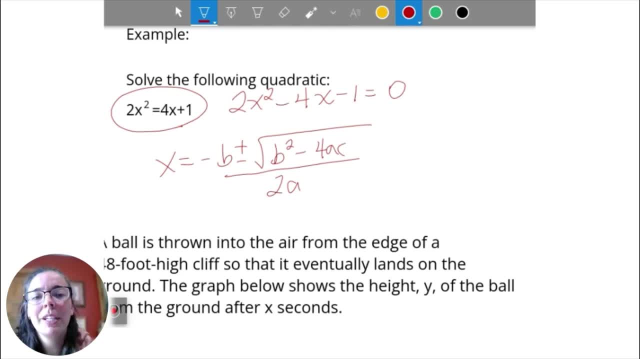 left. So I'm going to move everything over to the left. So I'm going to move everything over to the minus 4x. minus 1 equals 0. It needs to be equal to 0. That's key to find those solutions or those. 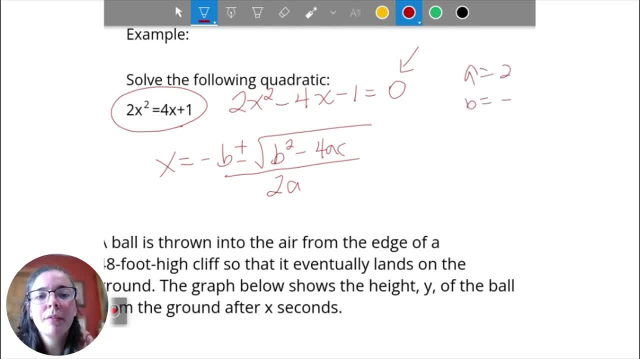 roots. So my a value is 2. b is negative, 4. c is negative, 1. Now, when I go and plug this in I you know what. I actually need a little more space, So let me give me a little more. 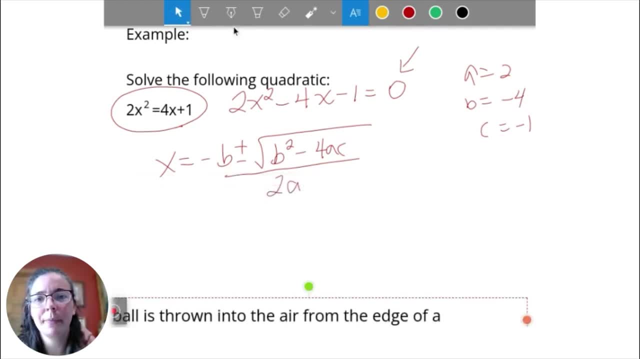 room here to do this. Okay, So let's go ahead and plug in. So we have: x equals negative, negative 4. right b is negative 4.. So we have to have negative negative 4 plus or minus square root of b squared minus 4.. The a is 2.. The c is negative 1, all over 2 times 2.. And now it's just a matter. 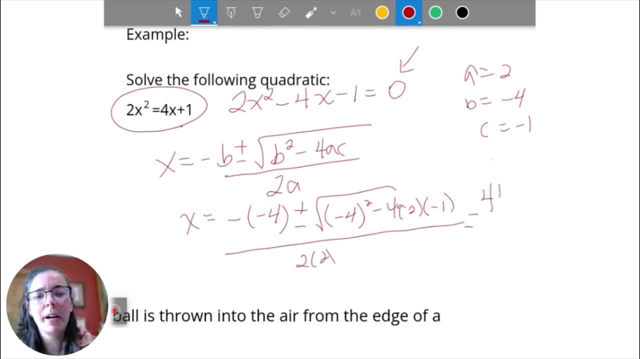 of simplifying. So negative, negative 4 is a positive 4.. Then what happens under my radical? So I'm going to use my calculator to simplify all of this stuff. So negative 4 squared minus 4 times 2 times negative 1. And you can break this up into different steps, if that's. 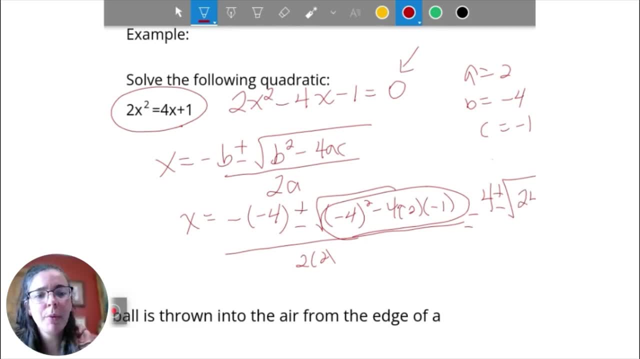 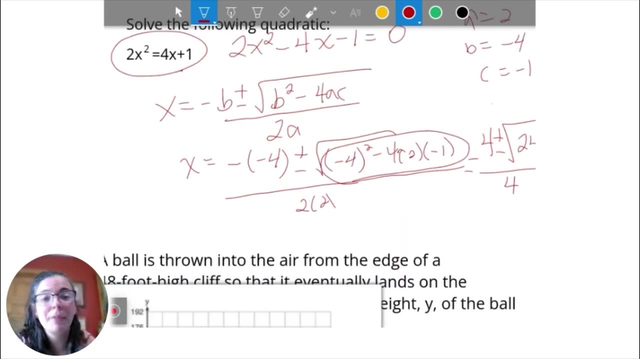 helpful for you. I'm just going to do it in one step And I get the square root of 24.. And this is all over 4.. So from here, the last thing I need to do is see: can I simplify the square root of 24?? 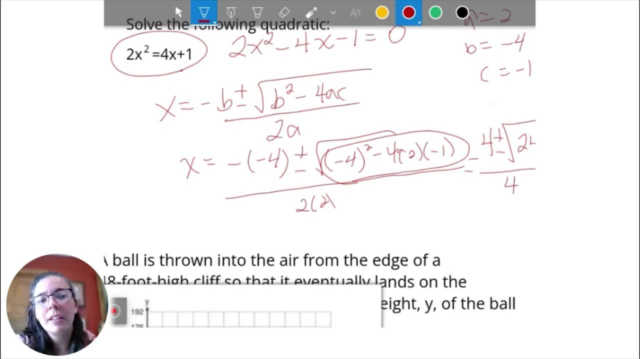 So the square root of 24 would be not a perfect square. So I just have to check: are there any perfect square factors of 24?? And actually 4 is 1.. So I'm going to use my calculator to simplify this. So I'm going to. 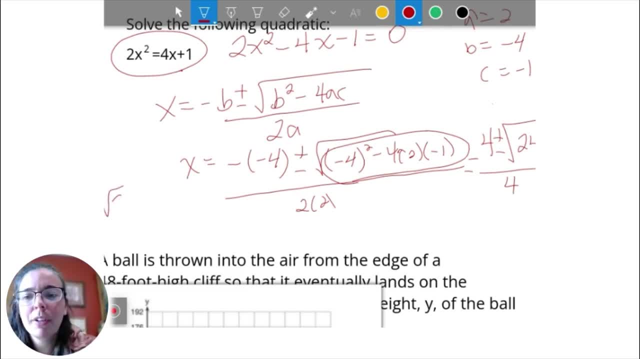 one of them. So off to the side here, let me just show you the square root of 24.. We can break into square root of 4 times the square root of 6. And square root of 4 is really just 2.. So this can. 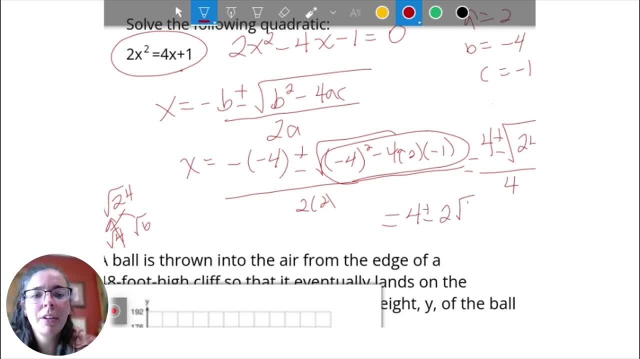 simplify to 4 plus or minus 2 square roots of 6, right, Because that's what's left over all over 4.. And to simplify that, you just get 1 plus or minus 2 over 4 is a half, And so this would: 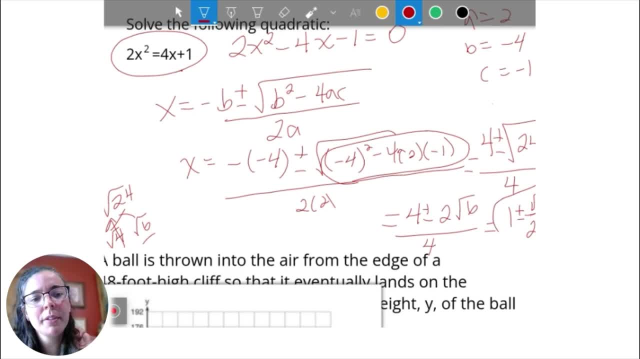 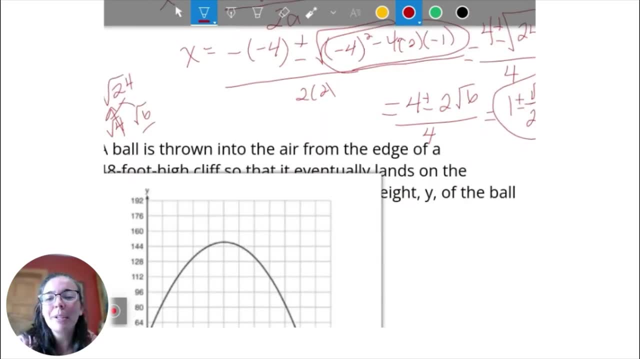 I could actually just write as the square root of 6 over 2.. So 1 plus or minus the square root of 6 over 2.. All right, so kind of a lot going on there when we use the quadratic formula. Happy to do another video if you guys want me to go a little more in. 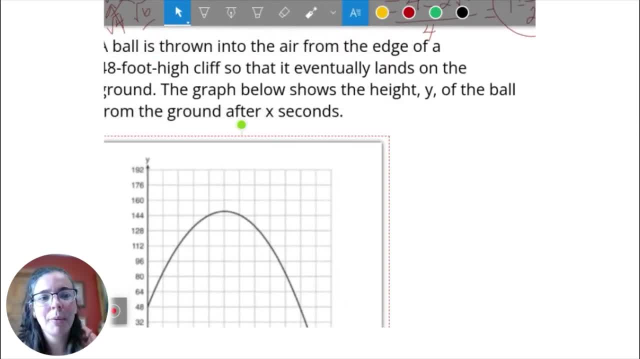 depth. All right, let's look at one application problem for quadratics as well. So a ball is turned into the air from the edge of a 48-foot high cliff so that it eventually lands on the ground. The graph below shows the height y of the ball from the ground after x seconds. 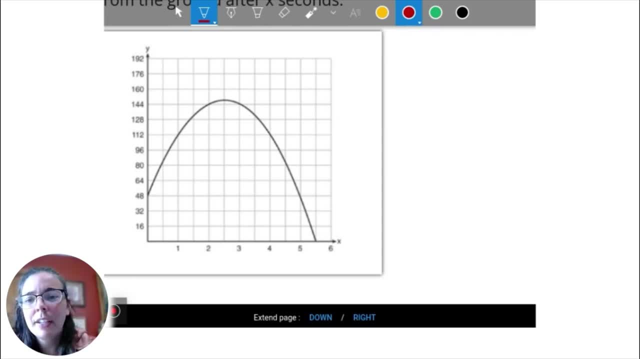 So here's our graph. It tells us it is at 48 feet on the cliff. So that's our 48 feet, right there our y-intercept. It goes up and then it starts to come down. So lots of questions that they could ask you here, For. 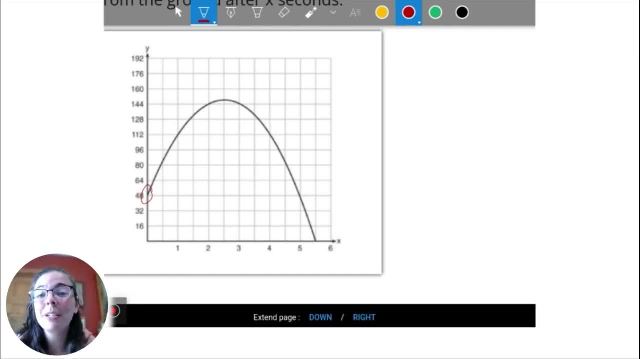 example, at what point does the ball hit the ground? So we need to be able to look at a graph and see what it means in relation to the problem. So if this is a ball, it's going up, up, up, up. 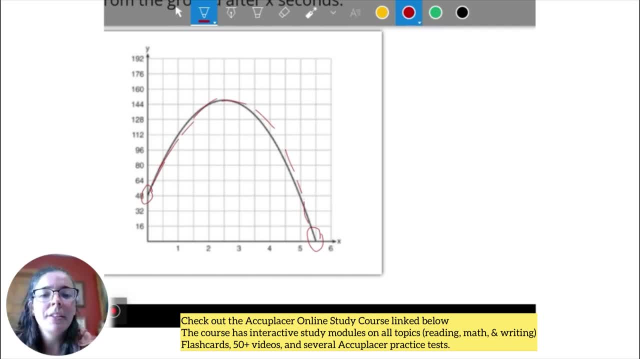 up coming down, down, down and down. It's going to hit the ground at a height of 0. So this would hit the ground when x is equal to 0. It looks like 5 and 1 half right. Another question they could ask you is: 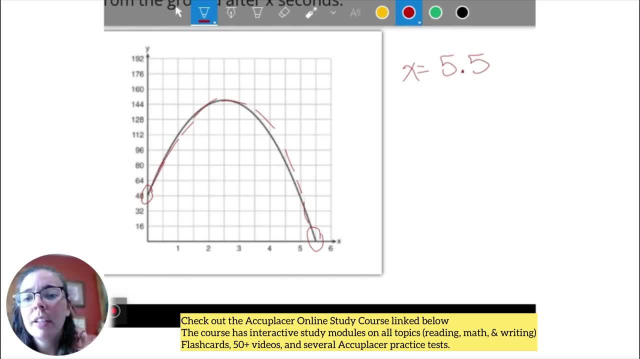 at what point is the ball at a height of 80?? So 80 is here. So at what height, or at what point, I'm sorry, is the ball at a height of 80?? Well, it looks like when we are at 1 half and 4 and 1. 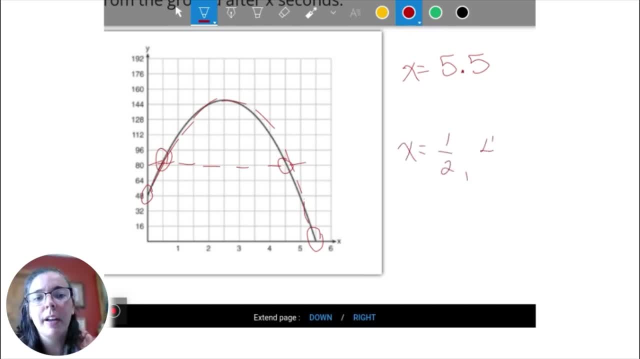 half. So that's when x equals 1 half, or 4 and 1 half. So lots of different questions they could ask you. We need to know how to look at a graph. So let's look at a graph. So let's look at a graph. 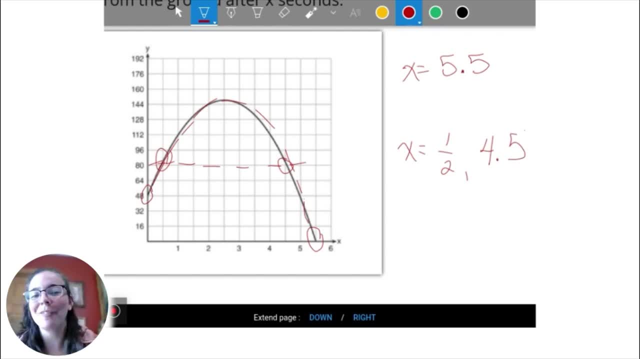 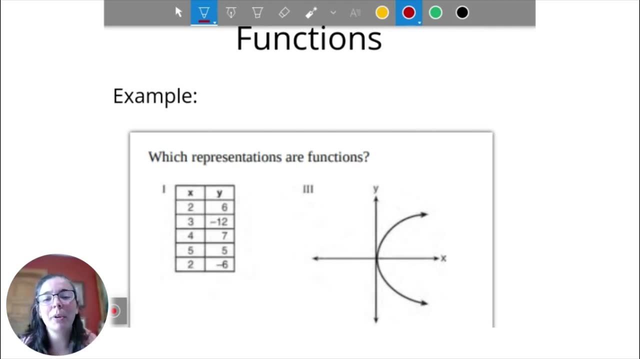 and pull out important information from that based on the question. All right, our next topic is functions. So functions are really important. You need to be able to see what is a function based off of a few different types of ways. they'll show it to you. 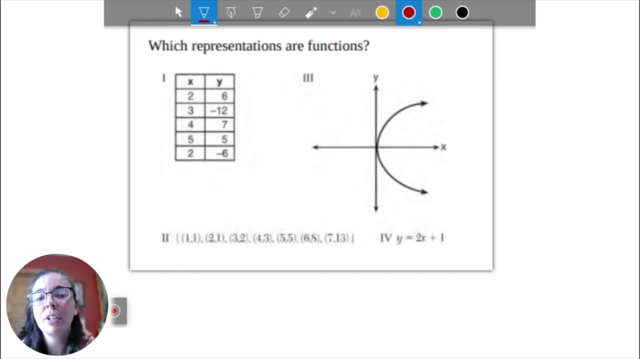 They may show it to you in a table, a graph, a set of coordinates or an equation. So which representations are functions? So function means that there are no repeat inputs, So the input is the x value. You need to make sure the x does not repeat. 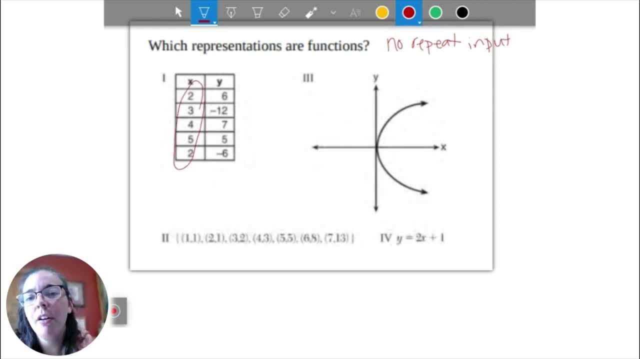 Okay. so if I'm looking at a table, does the x repeat here at all? Well, I do see two twice with two different y values. So that means that that is not a function. So number two: do I have any x's that repeat? It doesn't look like it. My y's repeat 1 and 1, but that's totally fine, That is. 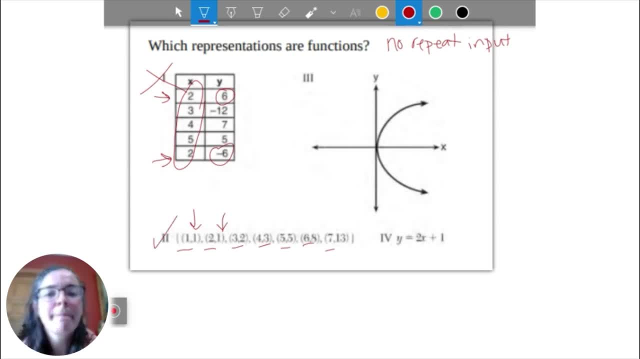 allowed, but our x is not, So that's fine. So if I look at a table, does the x repeat? here at all? cannot repeat, So this one works out. Three: is this a function? Well, now we don't have the actual. 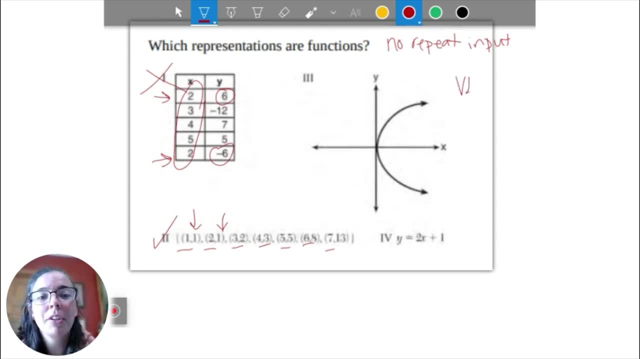 numbers or coordinates, but we can use what we call the vertical line test when we are using a graph, And that just means, if we draw a vertical line anywhere on the graph, if it hits more than once, which this does pretty much everywhere on the graph. 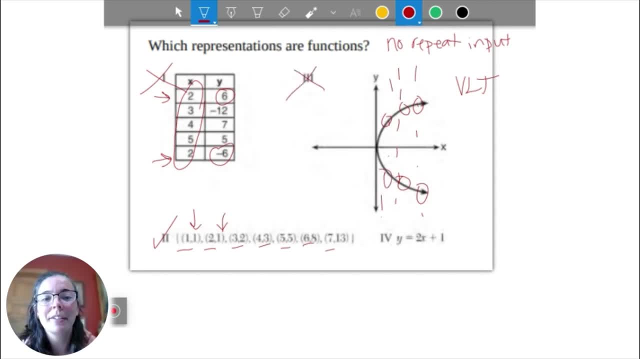 then it is not a function. So this does not pass the vertical line test. If you think about something like a line, a linear equation, this one would pass the vertical line test because it'll never hit more than once. Okay, And lastly, if you have an equation, y equals two x plus one. 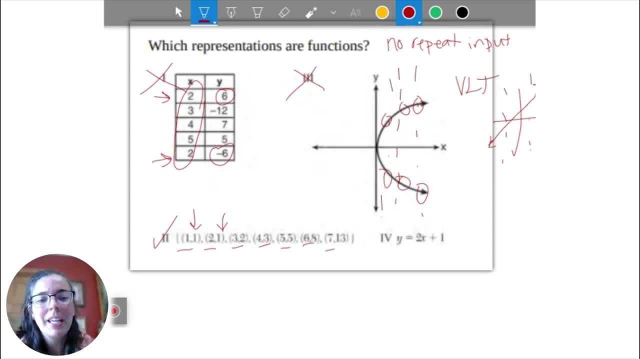 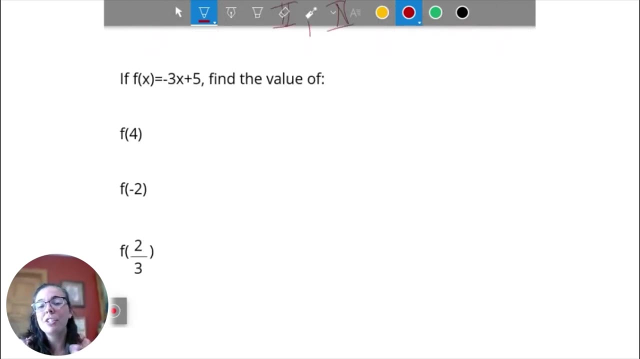 this would be a function, because any x value you plug in will give you a new y value. So our two functions are option two and option four. All right, And now another thing for functions is you have to be able to plug in and find the value of a function. So f of four, f of negative. 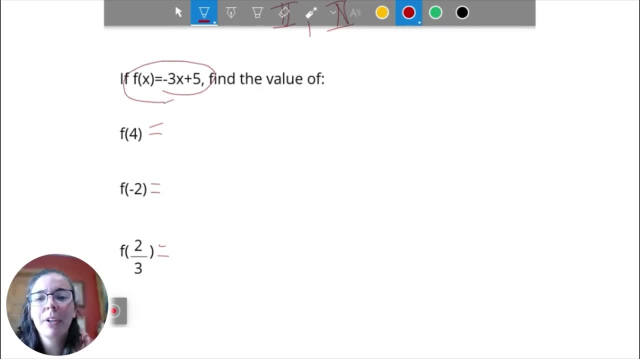 two and f of two thirds. we need to find those. if f of x equals negative three plus five, negative three, x plus five, So f of four would be negative three times four plus five. Negative three times four would be negative 12 plus five. That'll give me negative seven. All right, Maybe you can try. 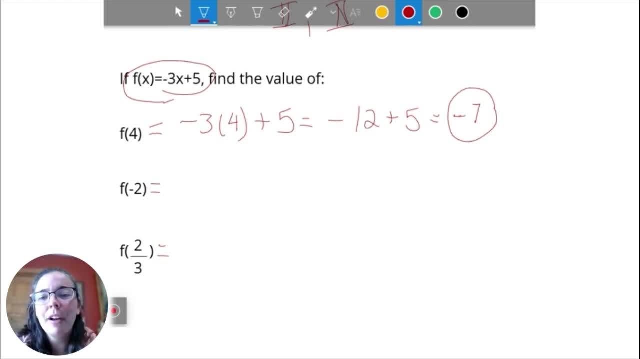 this next one. So maybe pause the video and let me know in the comments what do you get for f of negative three, Negative two. I'm going to plug in negative three times negative. two plus five. Negative three times negative two is six plus five gives me a positive 11.. And then one with a fraction, just because 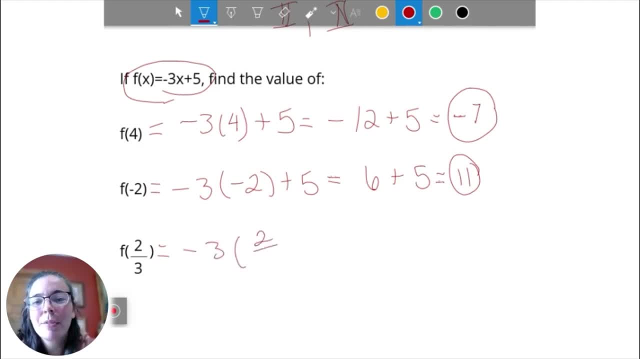 we all love fractions. Negative three times two thirds plus five. Well, negative three times two thirds. I can just multiply across the top and the bottom. Negative three times two is negative. six over three will just give me a negative two plus five. 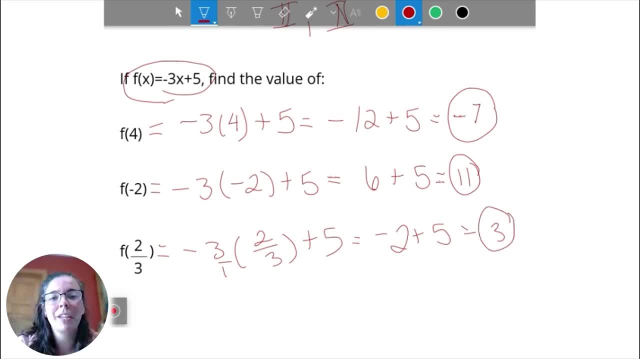 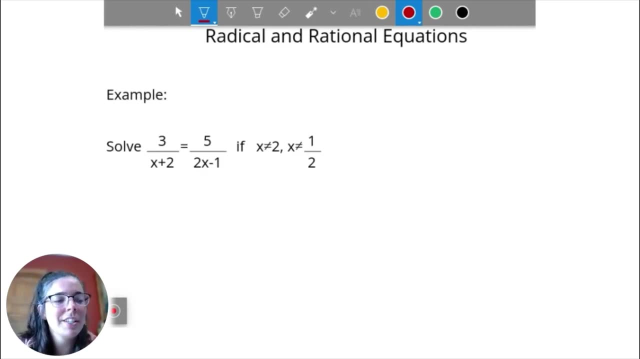 Which is a positive three. So there are a few things you need to know for functions for the ACCUPLACER exam. All right, Radical and rational equations is another thing we need to practice. So we need to solve maybe something like this: Three over x plus two equals five over two x. 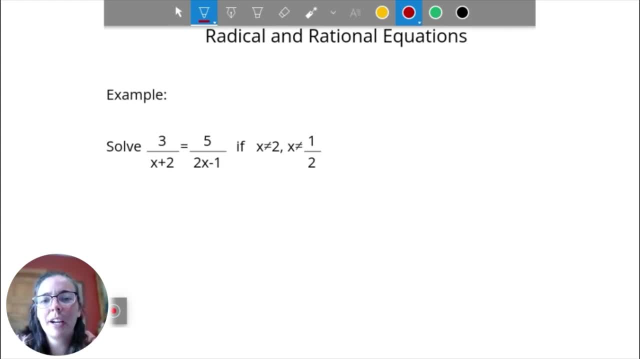 minus one, If x does not equal two and x does not equal one half. Actually, this should say: x does not equal negative two. Sorry, I think I had a typo there. X does not equal negative two And x does not equal one half. So if I'm trying to solve this, one way to do this would be to cross. 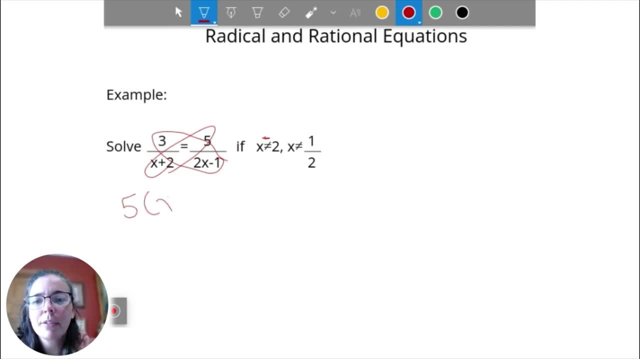 multiply. So five times x plus two has to equal three times two x minus one. So I'm going to distribute: five x plus 10 equals six x minus three, And in order to get x by itself, maybe I'll subtract five x from both sides And then add three to both sides. So I'm going to add three to both sides. 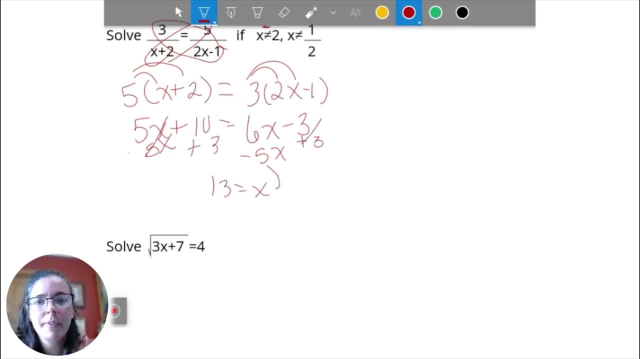 And I will get 13 equals x. So that is my value of x. that solves that equation. Now, how do we solve an equation with a radical? So this shows the square root of three: x plus seven equals four. So my goal is still to get x by itself. So, in order to undo the square root, we actually can. 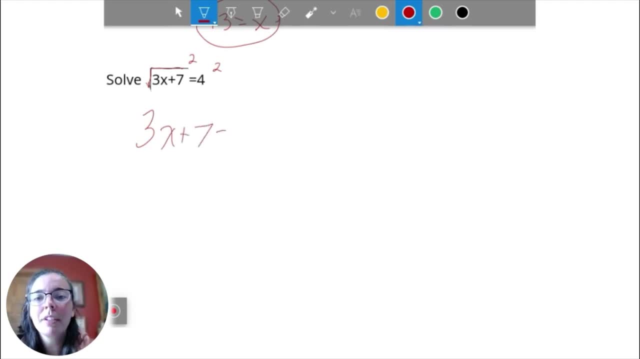 just square both sides, So that would leave me with three x plus seven equals 16.. And then I just have a pretty simple equation to solve: Three x equals 16 minus seven is nine, And when I divide by three I get x equals three. 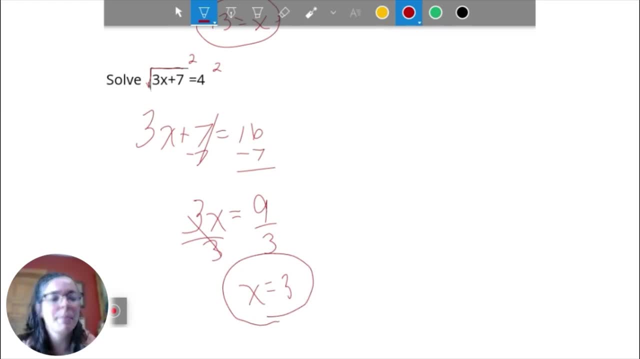 Right. So a couple examples of some radical and rational expressions, And we are moving right along to our next topic of polynomial equations. So let's solve something like this: Two x squared plus four x plus five minus three x squared plus four x minus 11 equals. 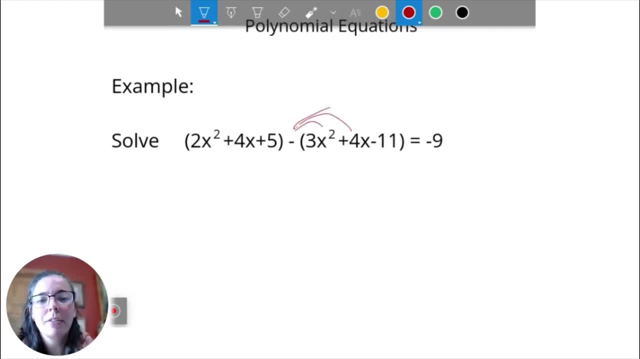 negative nine. So first thing is to get rid of this minus sign here. So we need to distribute this, So the first set of parentheses can just stay the same. But when I distribute this negative sign, I get negative three x squared minus four x plus 11. That equals negative nine. Okay, And then from: 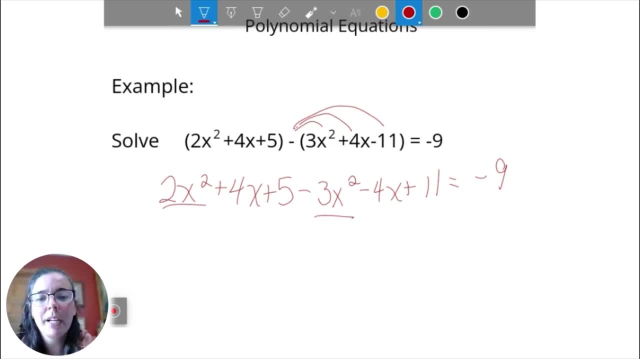 here. now I can combine some like terms: Two x squared minus three x squared is a negative. x squared Plus four minus four actually cancels out to be zero. And then plus five plus 11 is plus 16.. This equals negative nine. 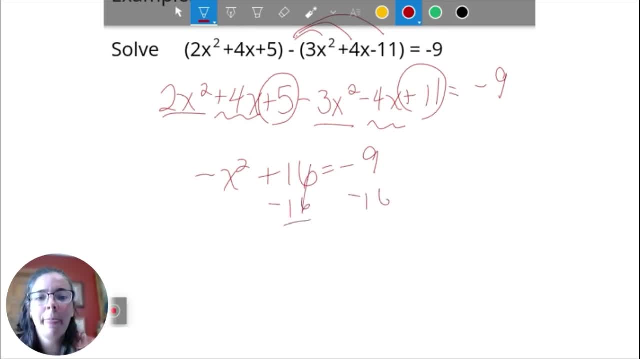 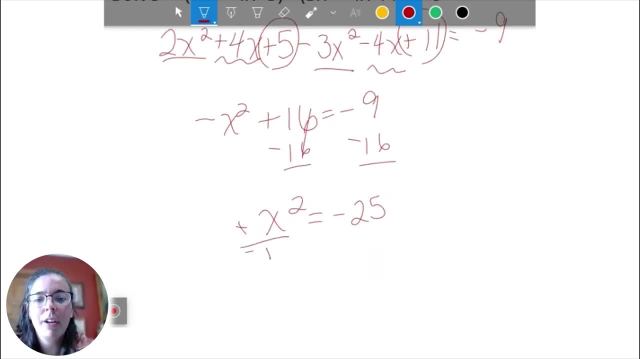 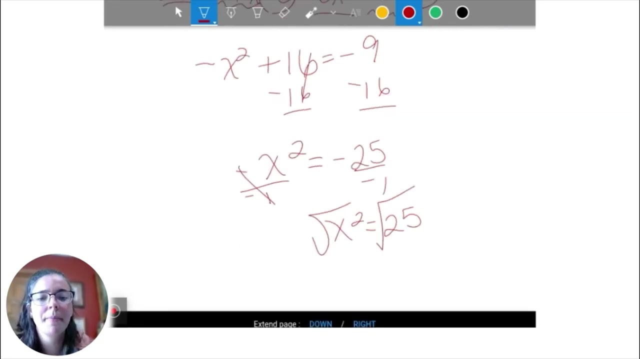 Now I will subtract 16 from both sides And I get x squared. Negative x squared equals negative 25.. Divide by negative one X squared equals a positive 25.. So the last step is to get rid of the x squared. I can just take the square root And I will get x equals. And it's important when we take 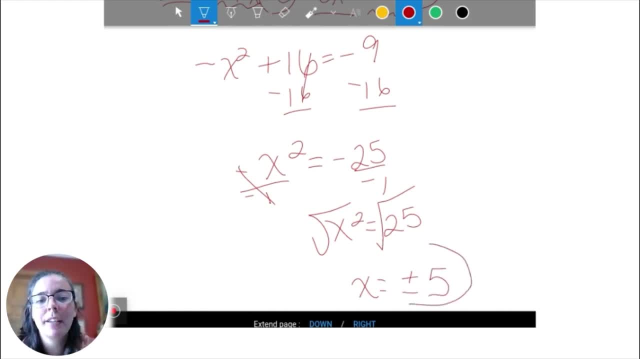 the square root of a number. the answer is either plus or minus the square root, which would be five. So our solution would be plus or minus five. So, solving polynomial equations, you may have to distribute a negative sign. combine like terms. 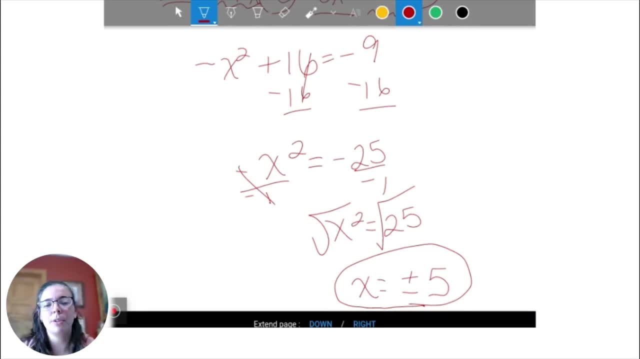 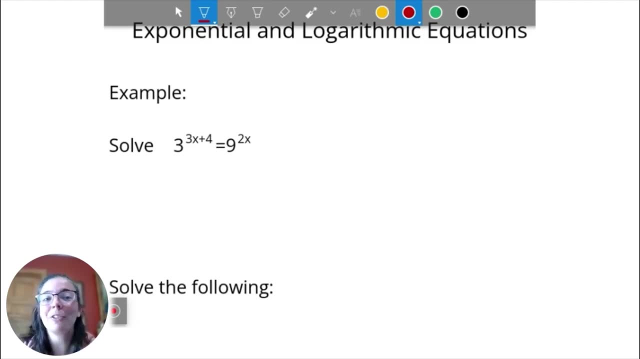 And then, at the end, you may need to take a radical like the square root or the third root in order to find a solution. All right, Exponential and logarithmic equations. So a few examples of things you need to know. Let's try to solve three to the three x plus. 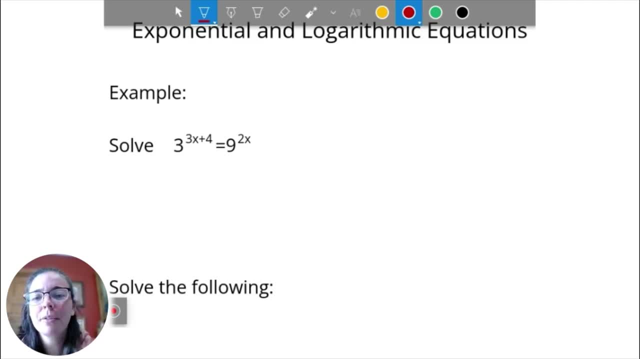 four equals nine to the two x. In order to do this we need the same base. So three to the three x plus four equals nine to the two x. So three to the three x plus four equals nine to the two x. So three to the three x plus four can equal nine, can be written as three squared. So this is the key. 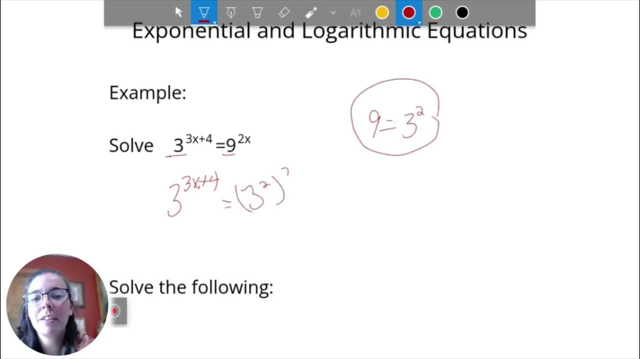 to this question. I can rewrite this as three squared to the two x, And then what that allows me to do is say three to the three x plus four equals three. Two times two x would be four x. So because I have the same base, the exponents must be the same. So three x plus four has to. 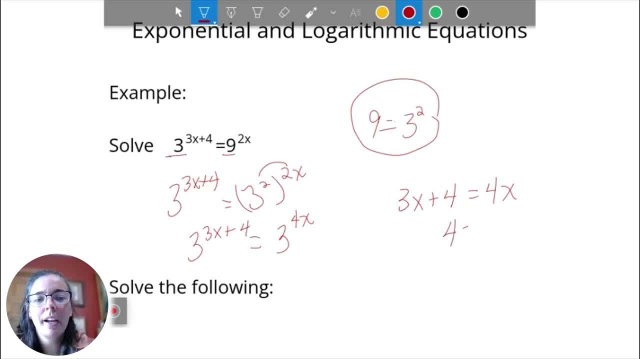 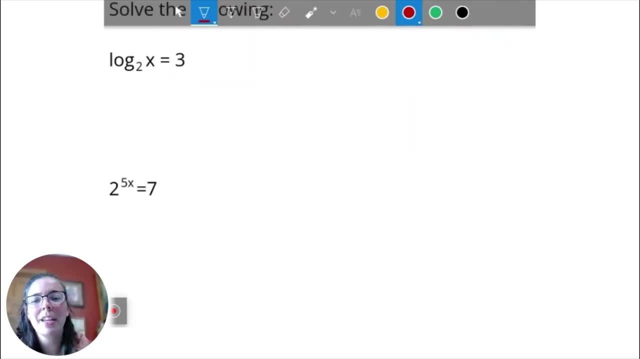 equal four x. And when I subtract three x from both sides, I get x equals four. So let's look at the equation. So let's look at the equation. So let's look at the equation. So let's look at the next example. Now we're going to take logarithms and go back and forth between exponential 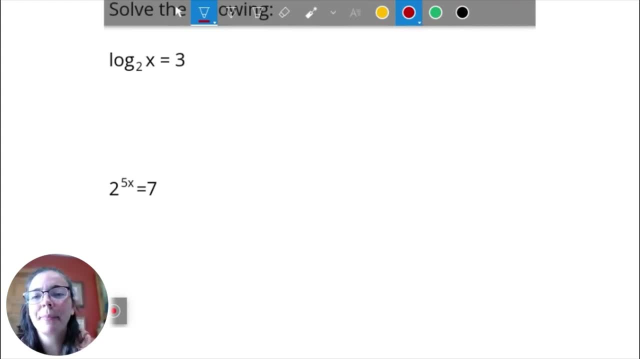 So let's solve the following: log to the base: two of x equals three. So in order to solve this and get the x by itself, I need to rewrite this as an exponential. So while I can do this, as the basis two and the exponent is always going to be what's on this side. So two to the third equals x And 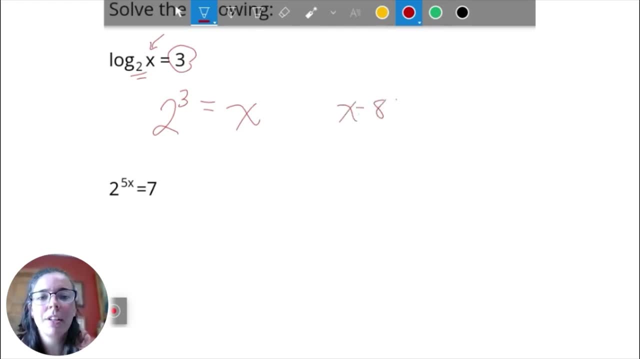 when I do two to the third, that is equal to eight. So this just is x equals eight And you could plug this in and check log base. two of x equals eight. So this just is x equals eight. And you could plug this in and check log base. two of x equals eight. So this just is x equals eight And you can plug. 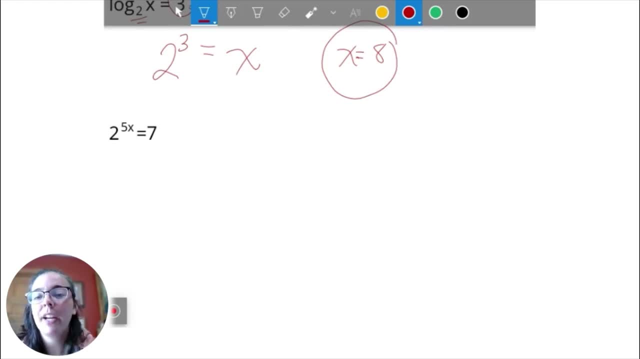 if I have an exponential and my variable is stuck up there and I need to solve for that variable, I can write this as a log. So log to the base: two of seven is going to equal five x. okay, So we could solve for that, And then I could just divide each side by five And I would find that x. 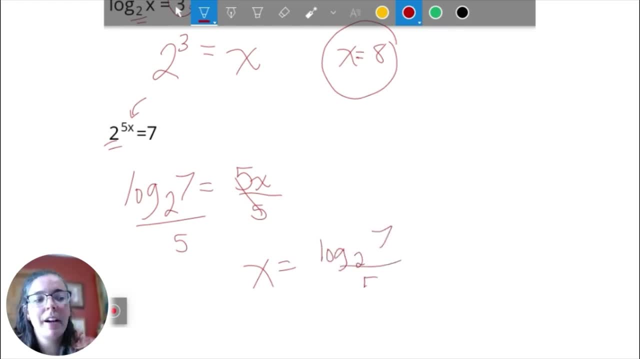 equals five x. So I just have to go back and forth between the spend and the spend So I can log to the log to the base 2 of 7 all over 5.. And say this is a multiple choice question. This is exactly. 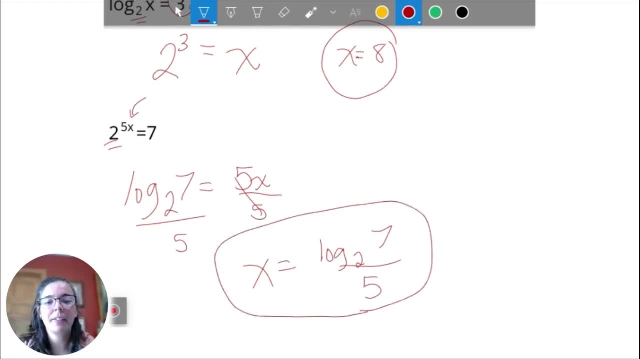 what your answer would look like. Okay so it's not pretty, it's not simple, but it is just a value where, if you had a graphing calculator or some higher functioning calculator, you could plug this in and get the value of that. Okay, so it's important to know how to convert back and 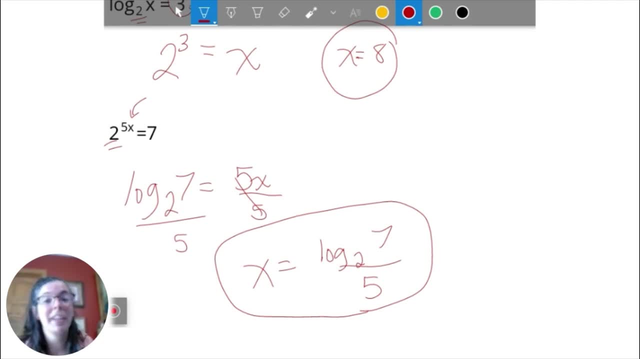 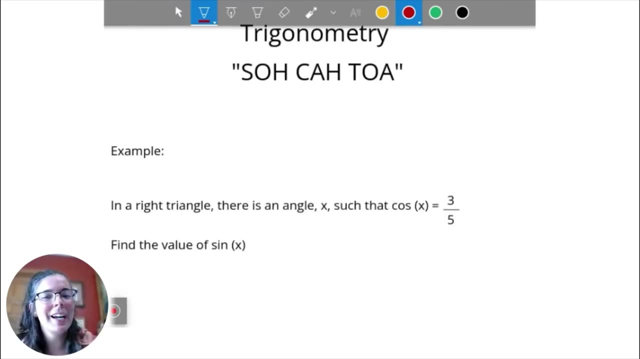 forth between logarithms and exponentials. So, again, if that's something that you're like, hey, pause the video right there. I need some more help. leave me a comment and I will make a new video about that. Okay, and we have our last topic. We're running out of time a little bit, so 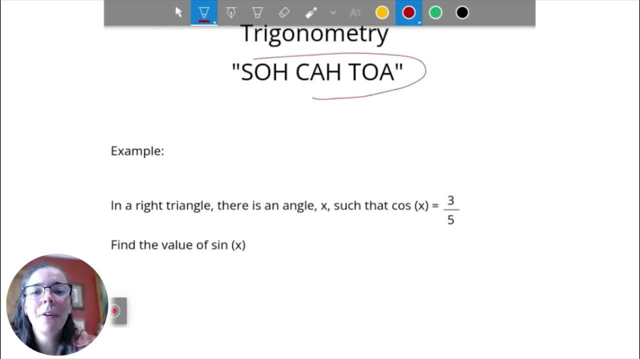 I'm going to fly through some trigonometry. Then one thing I really want you to know and have memorized is SOHCAHTOA. So SOHCAHTOA, what does that mean? Well, that is our three main functions, sine, cosine and tangent, And with trigonometry, a lot of times we're talking 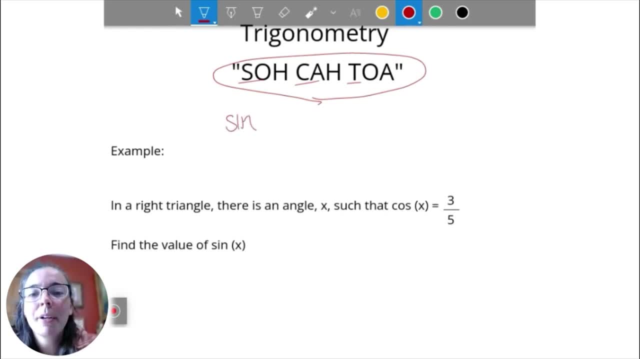 about right triangles and that helps us remember the sine, cosine and tangent Function. so sine is going to be the opposite side over the hypotenuse, Cosine is going to be the adjacent side over the hypotenuse And then tangent is going to be the opposite side over the. 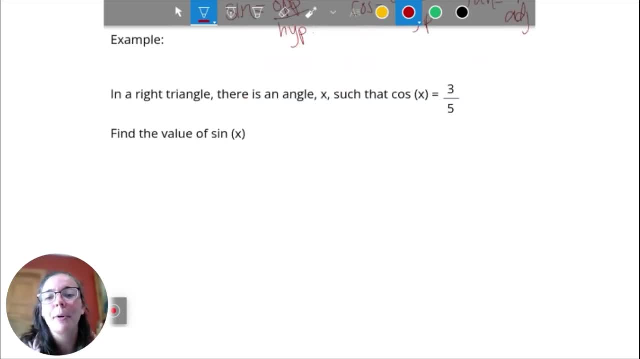 adjacent side. So what does that mean? Let's look in an example. In a right triangle there is an angle x such that cosine of X equals 3 over 5, find the value of sine X. So if I have a right triangle and I subtract and multiply the right triangle by sine, then I can let mu of x equal. 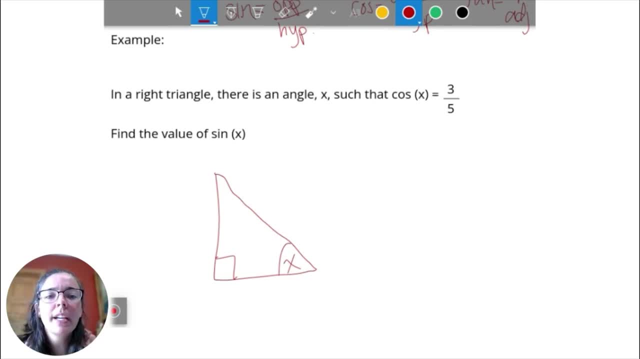 say this is x. okay, If cosine of x equals 3 over 5, well, so, katoa, this is adjacent over hypotenuse. So that means that 3 is my adjacent side and my hypotenuse is 5.. So I need to find the sine. So 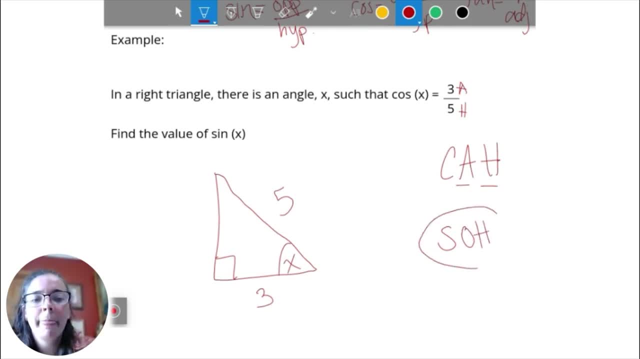 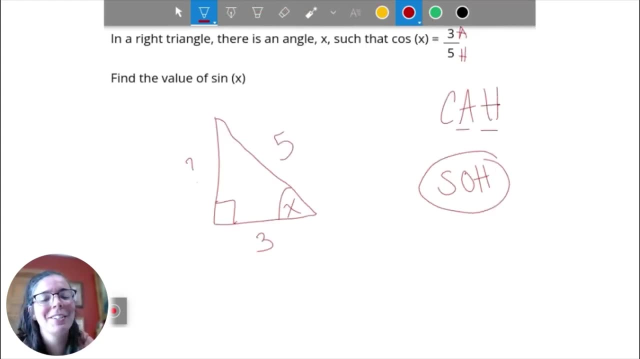 the sine of x is going to be so opposite over hypotenuse. So I need to find this in order to find the sine. Now, from your geometry skills, we know how to find the side of a right triangle by using the Pythagorean theorem. See if that rings a bell. a squared plus b squared equals c squared. 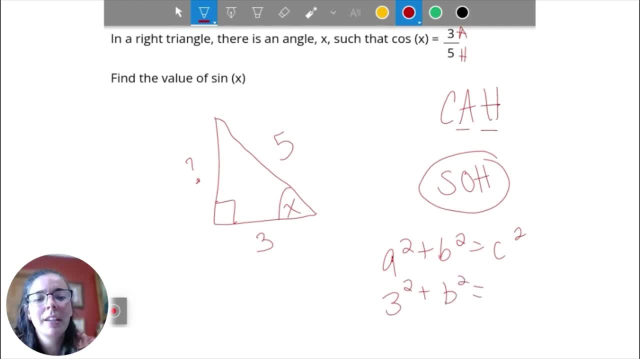 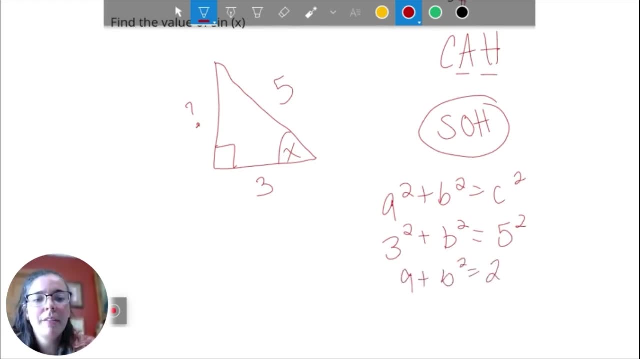 So I can just plug in what I know: 3 squared- I'll solve for b- equals 5 squared, So I get 9 plus b squared equals 25.. Subtract 9 from both sides, b squared equals 16.. And when I take the square, 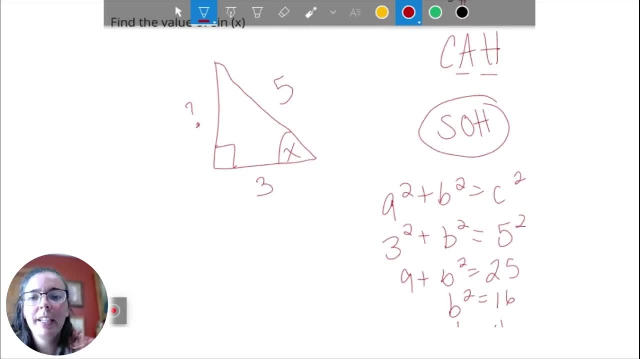 root, I get b equals 5.. So I get 9 plus b squared equals 25.. Subtract 9 from both sides, b squared equals 4.. So that's the value I needed to help figure out the sine of x, which is the opposite. 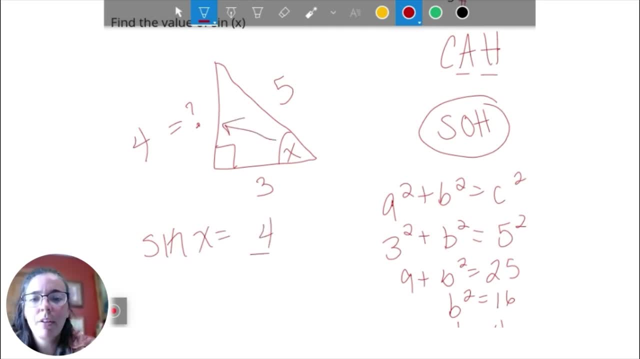 side, right across from it, over the hypotenuse, which is always across from the right angle, the longest side, And my value would be 4 over 5,. okay, So we did a lot of examples in this video today. I hope you found them helpful And if you want more practice like this, make sure you check. 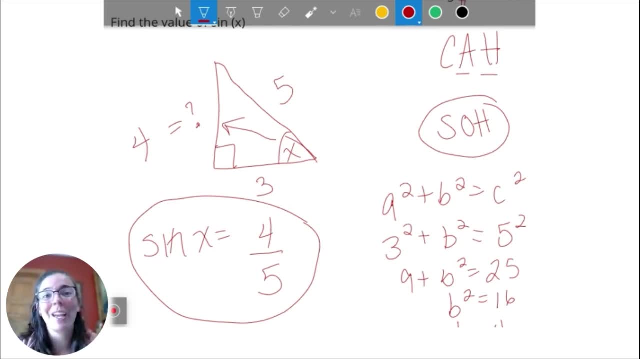 out the links in the description of this video For our online practice. we have a link in the practice test which you can get for free at Smart Edition Academy, as well as our full online course, So I hope this helped. Check out our other videos for the ACCUPLACER exam. We will have more.